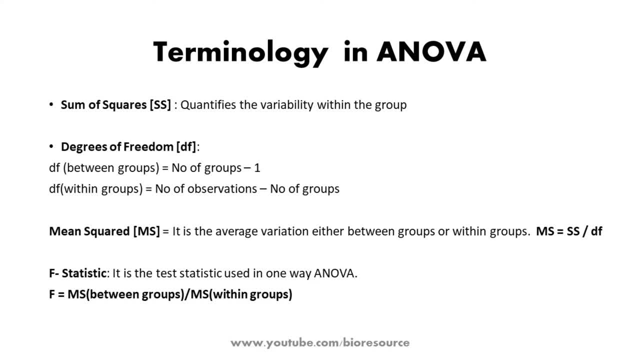 and degrees of freedom within groups, between groups and within groups. So for degrees of freedom within between groups is calculated number of groups minus 1 and degrees of freedom within groups is equal to the number of observation minus the number of groups and coming to mean squared, it is the average variation either between groups or within the groups. 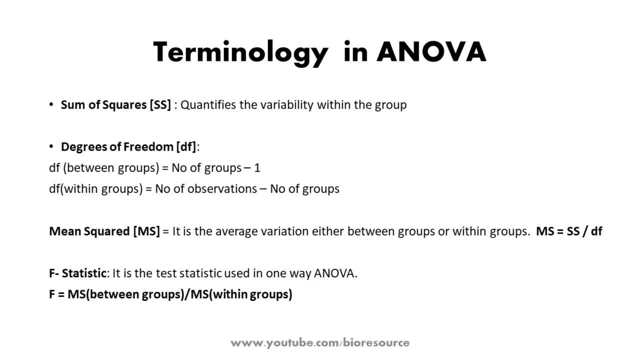 So mean squared is calculated by taking the ratio of sum of squared and the degrees of freedom and f-statistic. it is the test statistic used in one-way ANOVA and it is calculated by taking the ratio of mean squared between groups and the mean squared within groups. 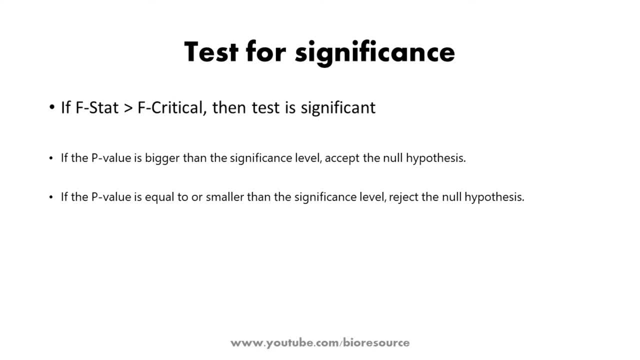 and the test for significance. if f-statistic is greater than f-critical, then the test is significant, and if the p-value is bigger than the significance level, then we will accept the null hypothesis. and if the p-value is equal to or smaller than the significant level, then we will 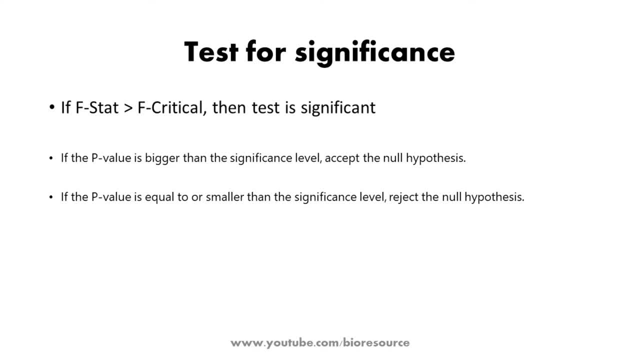 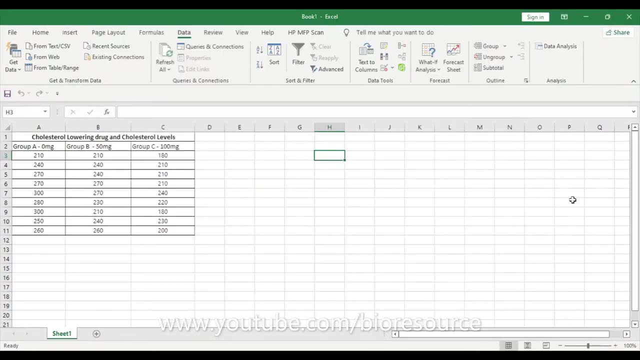 reject the null hypothesis. So this is all about the ANOVA and the terminology or basic introduction to ANOVA. Now let's see the real example using a cholesterol data. Now let's see the real data. here we have three different groups with different drug dosage. 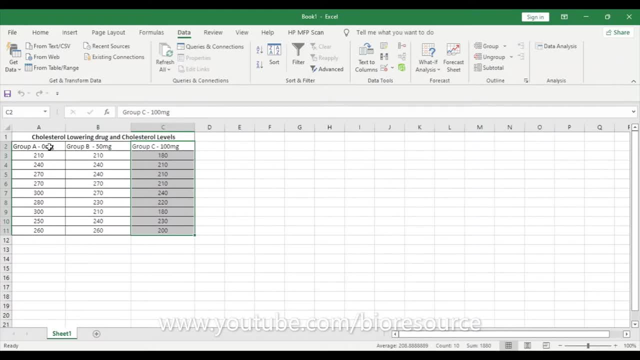 taken. These are the cholesterol lowering drug. group A received 0 mg, so they did not receive. these are the control groups. group B received 50 mg of the drug and group C received 100 mg of the drug, and the cholesterol measurements of each group is measured. and now let's see. 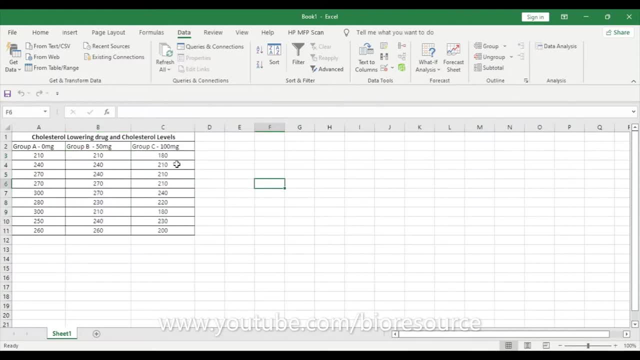 what is the effect of the cholesterol lowering drug in the cholesterol levels of these individuals? So to do the one-way ANOVA we have to use data analysis- data analysis back. I will show you how to enable this. if it is not already present, click on. 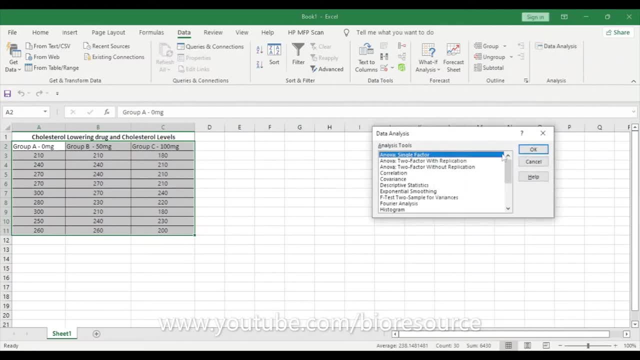 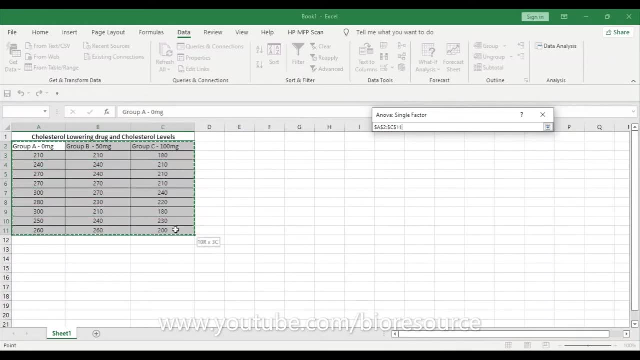 the data analysis and do a single factor ANOVA and click OK. now we will get the input range. so select the heading along with the cholesterol data group by. if the data is grouped by column, select column. otherwise use rows. and if you have selected the labels, tick this box saying that labels in the first row. so 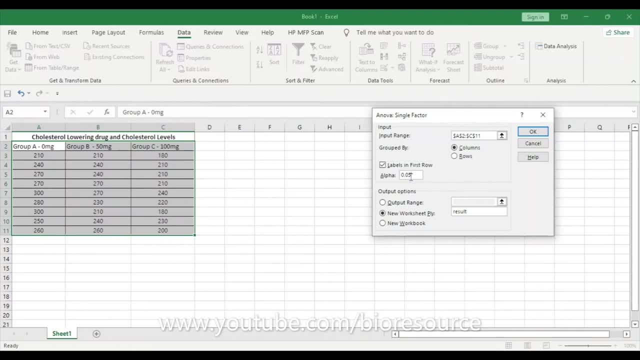 this is for the alpha and our alpha is: this is a significant level, that is, 0.05, and we want the output whether in the same range or in the new worksheet. so I have given in the new worksheet with result as the sheet name. now click OK. so 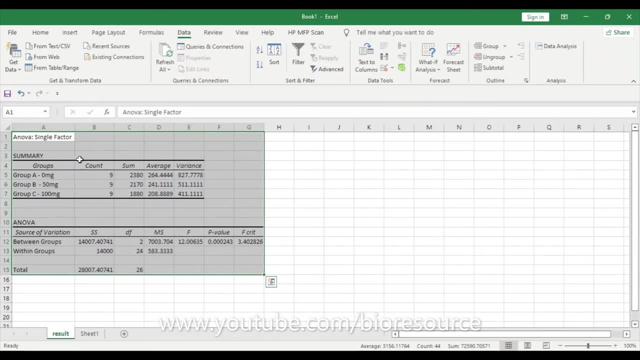 now we have the two tables here. one is the summary table and the other is the ANOVA table. the summary table has three different groups, data, that is, group A, group B and Group C, and count of each group. so nine measurements are there from each group. 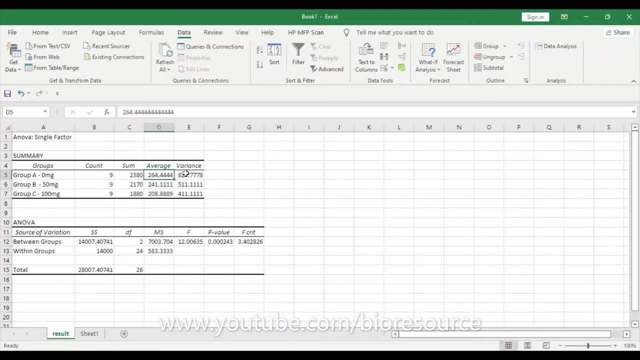 and the sum, total sum and the average and the variance. so variance is the average of square difference from the mean and it is a measurement of spread between the numbers in the data set. so we have variance, average sum and the count of three different groups. now coming to the anova table. so we have here source of variation between groups. 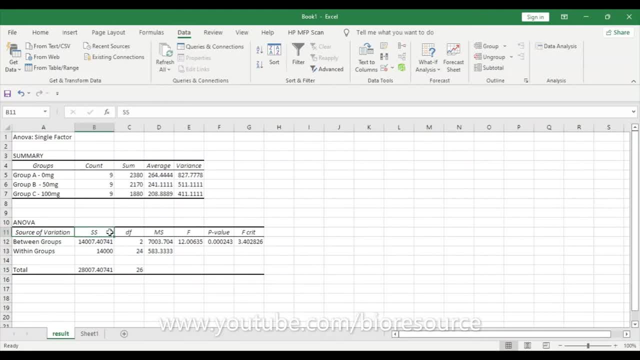 and within the groups, and the first one is the sum of squared. sum of squares is: it quantifies the variability within the group, and df is the degree of freedom. so degree of freedom between groups is calculated by number of groups minus one, that is two. so three groups are there three? 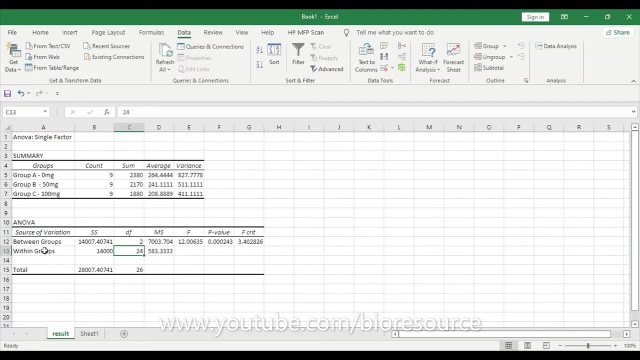 minus one is two, and the degrees of freedom within groups is calculated by taking number of observation minus number of groups. so here total observations are 9 plus 9 plus 9, that is 27, subtracted by the number of groups, that is 3. so total degrees of freedom within the group is 24..